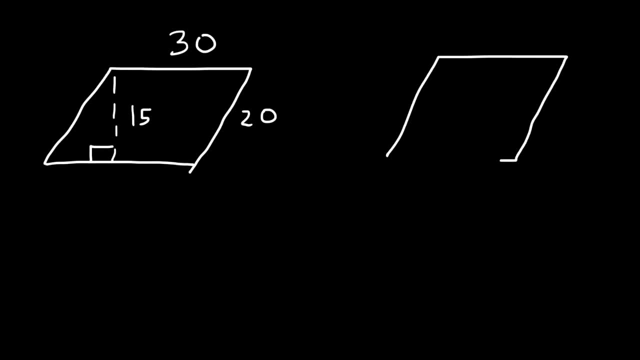 All you need to find. the area of a parallelogram is the length of the base and the height, also known as the altitude. So the area is simply base times height. In this example, the base is 30, and the height is 15.. 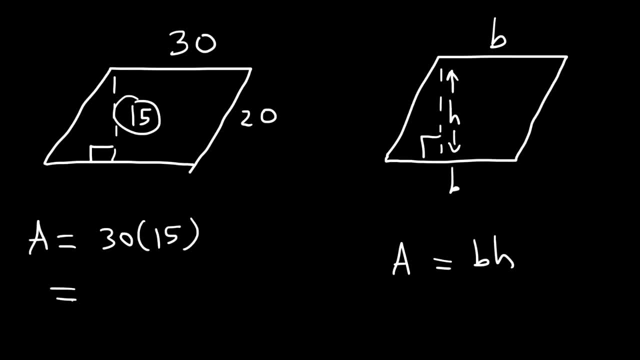 So it's just 30 times 15.. 30 times 15 is about 450.. And so that's the area for this example. Let's work on some more examples. Find the area of this particular parallelogram, So it has a base of 20, and a height of 25.. 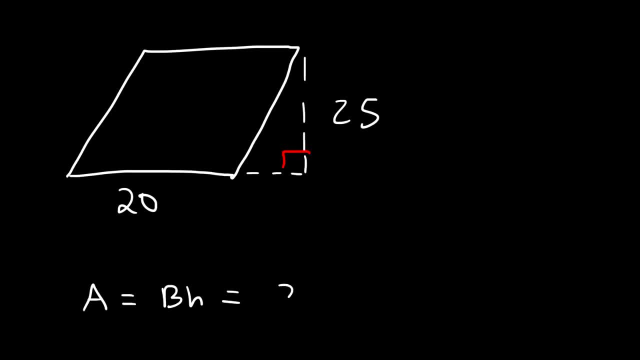 So the area is simply base times height, 20 times 25. And that's going to be 500.. So it's 500 square units, And that's basically all you need to do to find the area of a parallelogram. 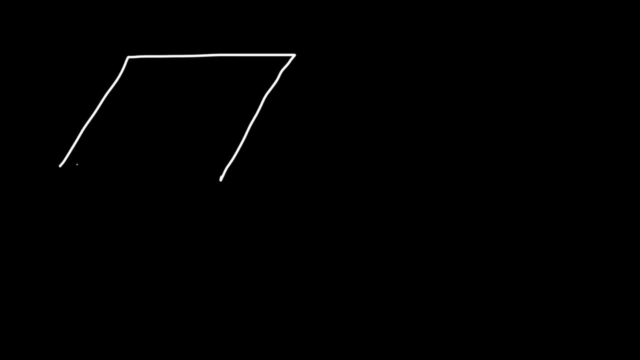 Let's work on one more example. Let's work on one more example. So let's say that this side is 11.. These two sides are 13.. And let's say that this side here is 6.. Find the area of the parallelogram. 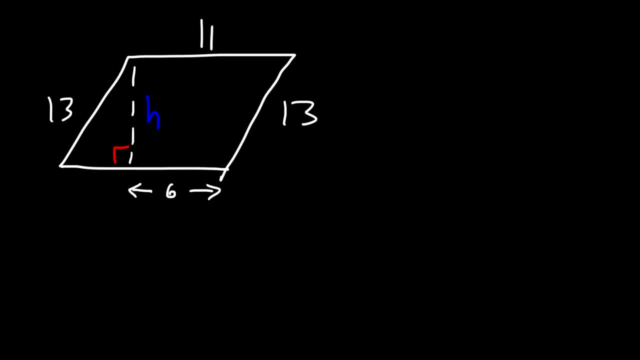 What we need to do is we need to find the height. Now, if this side is 11,, then this side must also be 11.. 11 minus 6 is 5.. So this section is 5.. Now let's focus on the right triangle that we see here. 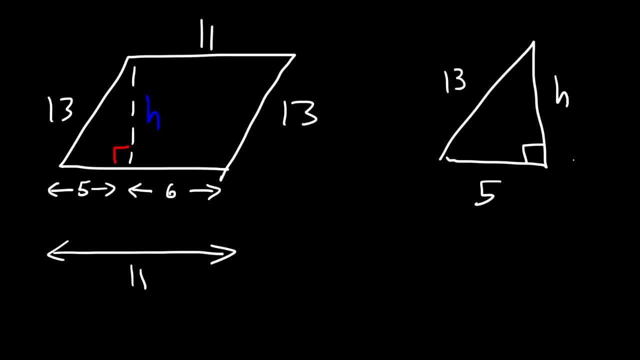 This side is 5.. This side is 13.. We need to find the missing side. So we can use the Pythagorean theorem: a squared plus b squared is equal to c squared. Let's say a is 5, b is the height and c is 13..